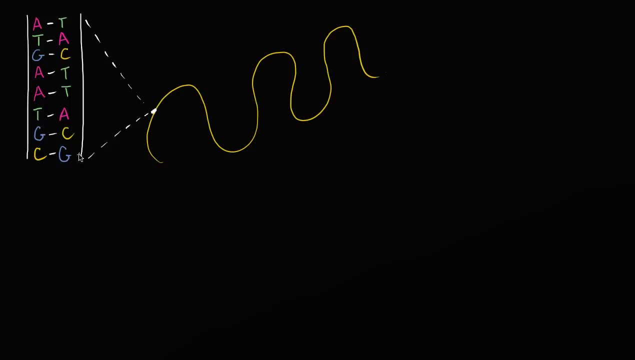 As a cell divides, the two new cells would want to have the same genetic material. So how does DNA replicate? And this process is called replication. So let me replication- and we covered this in the introduction video as well, but it's nice to see the different processes. 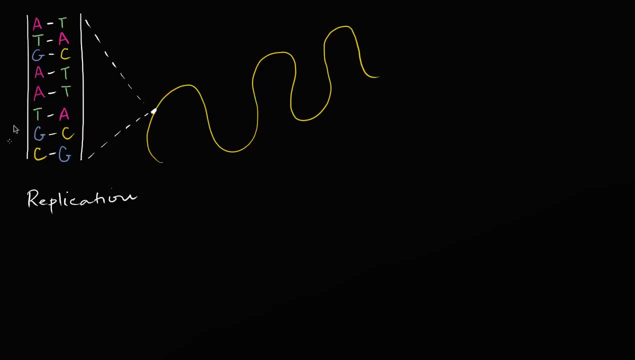 next to each other And replication. well, you can imagine taking either both splitting these two sides of the ladder, and actually let's do that, So let me copy and paste, So if I take that side right over there, and so let me copy and then paste it. 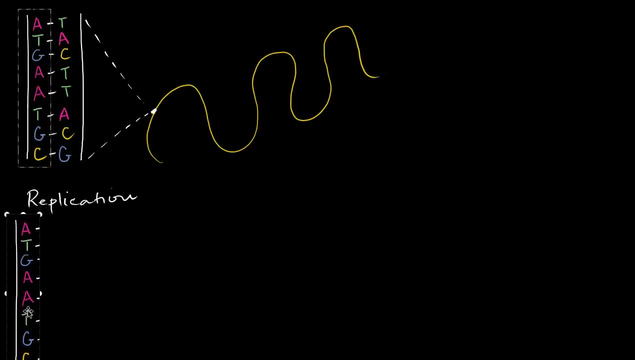 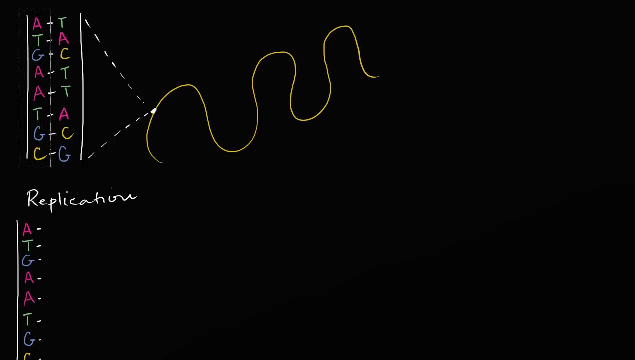 And then there we go. A little bit of it is dropping below the video, but I think that serves the purpose. And then, and then let's copy and paste the other side. So let me select that, And then I copy, and then I paste. 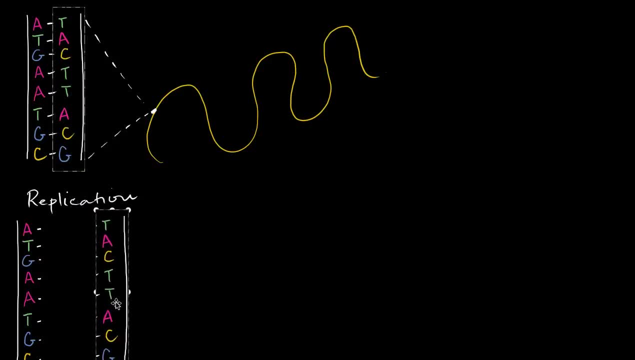 And it's just like that. And so you can imagine if you were to split these, these- I guess you could call them two sides of the ladder- then either side could be used to construct the other side, and then you would have two strands. 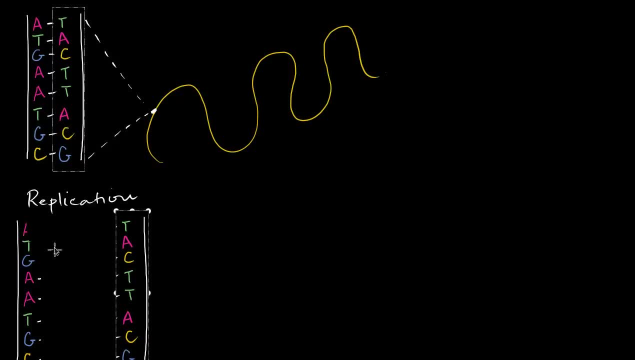 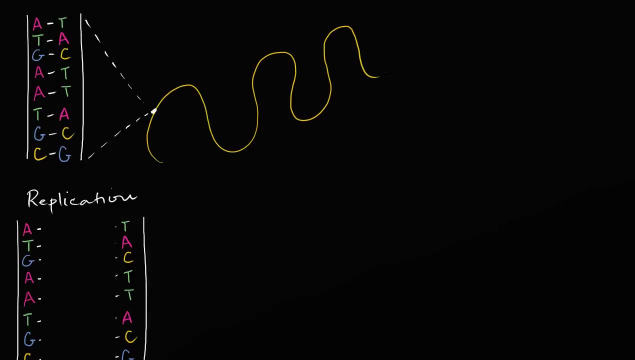 two identical strands of the DNA, And so let's see what that actually looks like. So let me get my pen tool out now. Let me deselect this Pen tool out. it's a new tool I'm using, so let me make sure I'm doing it right. 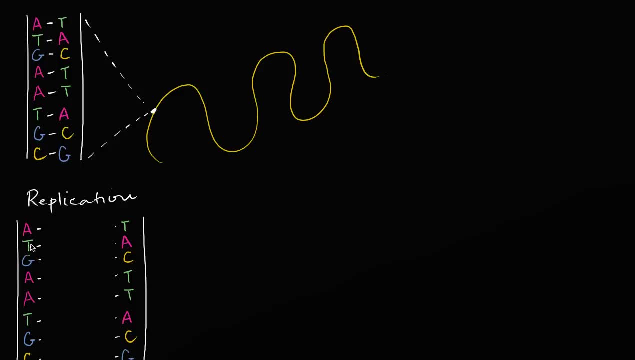 All right. so from this side, from this left side- or at least what we are looking at is the left side- you can then construct another right side based on this information: A always, always, pairs with T if we're talking about DNA. 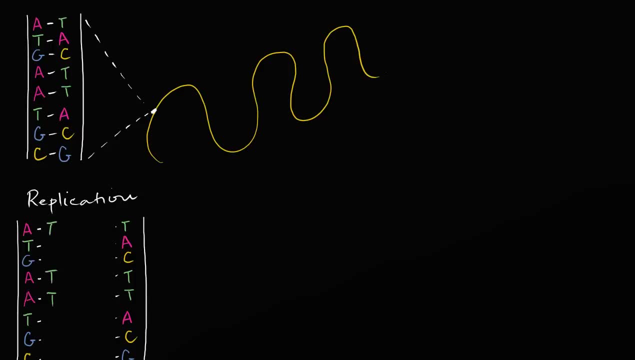 So adenine pairs with thymine, just like that Thymine pairs with adenine. Let me do that a little bit neater: Thymine pairs with adenine, Guanine pairs with cytosine. That's cytosine, cytosine pairs with guanine. 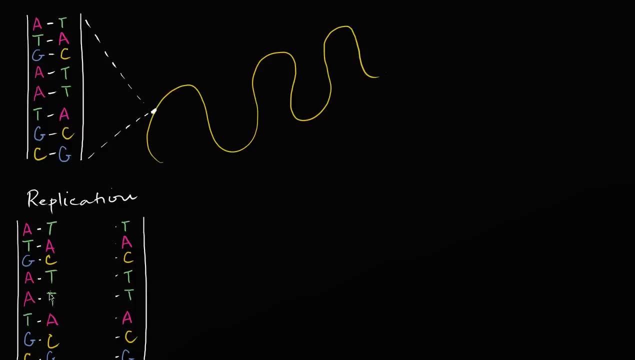 falling a little bit down here And just like that I was able to construct a new right-hand side using that left-hand side. So maybe I'll do the new, the new sugar phosphate backbone in yellow, And we could do the same thing here. 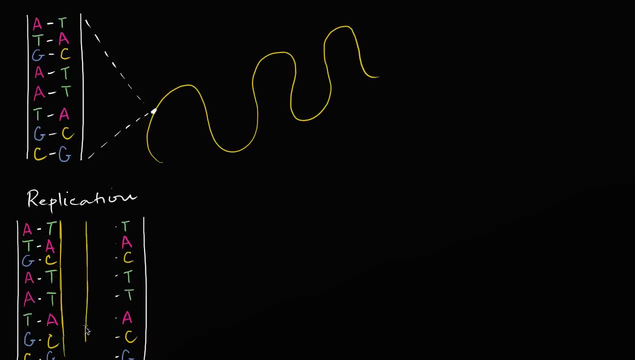 using the original right-hand side. So using the original right-hand side once again. the Ts pair with the As thymine- let me do that- and that adenine's color, so we have an adenine and thymine. 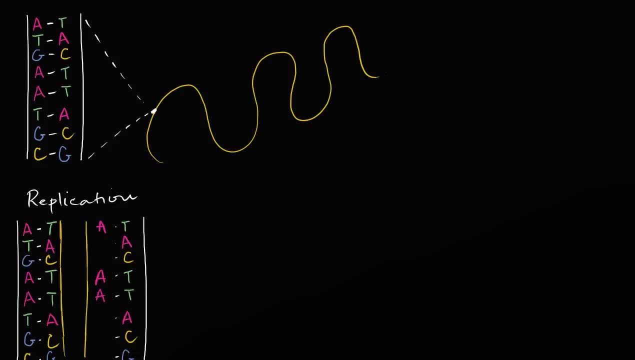 adenine and thymine. adenine and thymine, Thymine pairs with adenine, so thymine adenine, Thymine adenine, Guanine pairs with cytosine, Guanine, guanine. 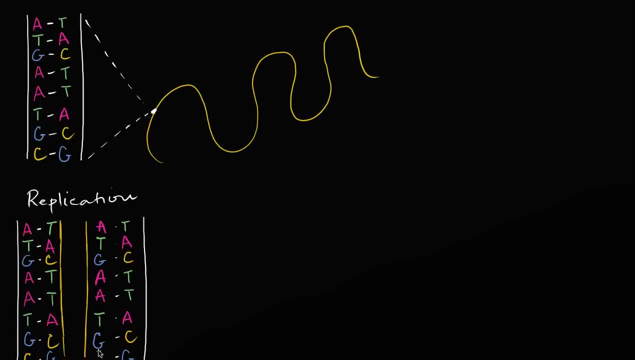 And then cytosine pairs with guanine, So cytosine, just like that, And so you can take half of each of this ladder, and then you could use it to construct the other half, and what you've essentially done is you've replicated. 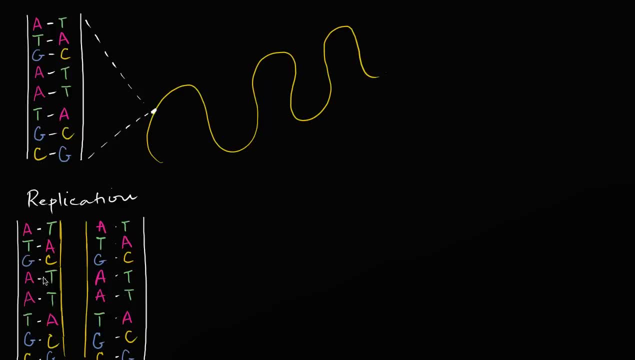 the actual DNA. And this is actually a kind of conceptual level of how replication is done before a cell divides and replicates and then the entire cell duplicates itself. So that's replication, So the next thing you're probably thinking about. okay, well, you know, it's nice to be able. 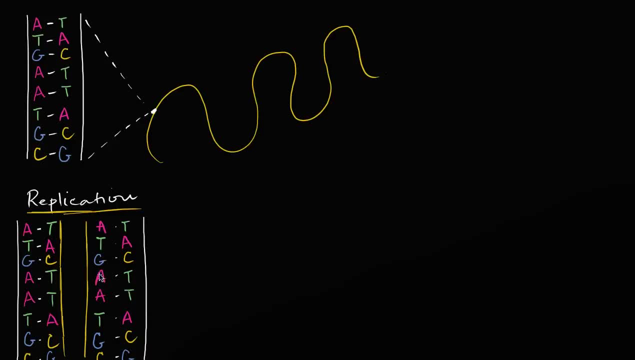 to replicate yourself, but that's kind of useless if that information can't be used to define the organism in some way, to express what's actually happening. And so let's think about how the genes in this cell, in this DNA molecule, are actually expressed. 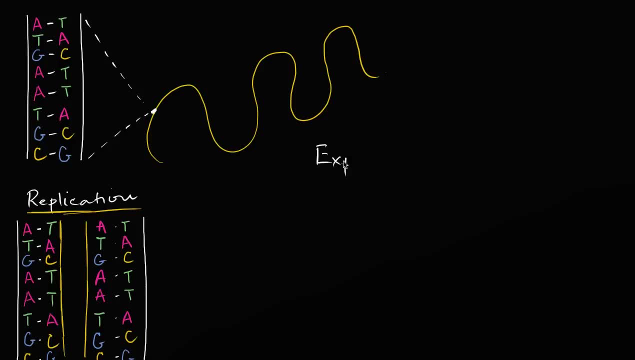 So I'll write this as expression Expression, And actually that actually warrants a little bit of a detour, because you hear sometimes the words DNA and chromosome and gene used somewhat interchangeably and they are clearly related, but it's worth knowing. 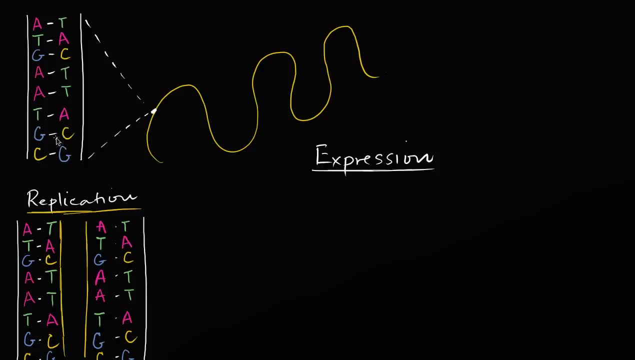 what is what? So when you're talking about DNA, you're talking literally about this molecule here that has this sugar-phosphate base and it has these sequence of base pairs. It's got this double helix structure And so this whole thing, this could be a DNA molecule. 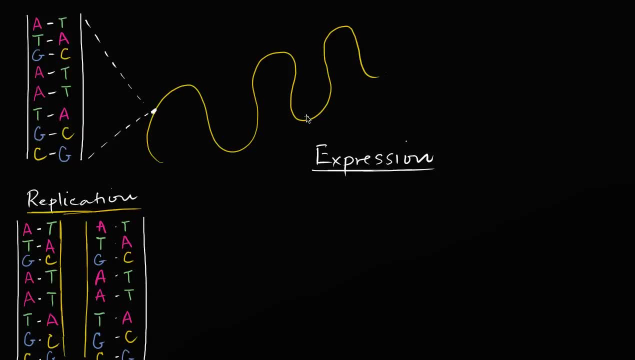 Now, when you have a DNA molecule that's packaged together with other molecules and proteins and kind of given a broader structure, then you're talking about a chromosome, And when you're talking about a gene, you're talking about a section of DNA that's used to express a certain trait. 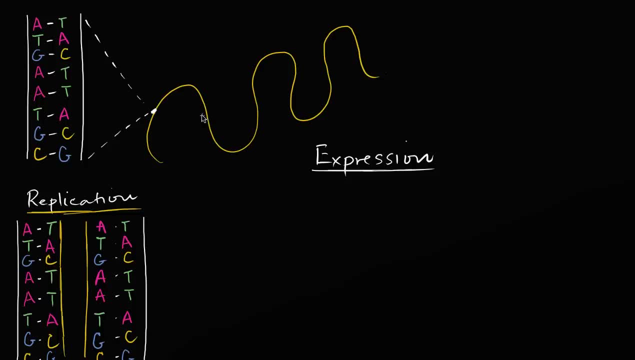 or actually used to code for a certain type of protein. So, for example, this could be, this whole thing could be a strand of DNA. but this part right over, let's say in orange, I'll do it. this part in orange right over here could be one gene. 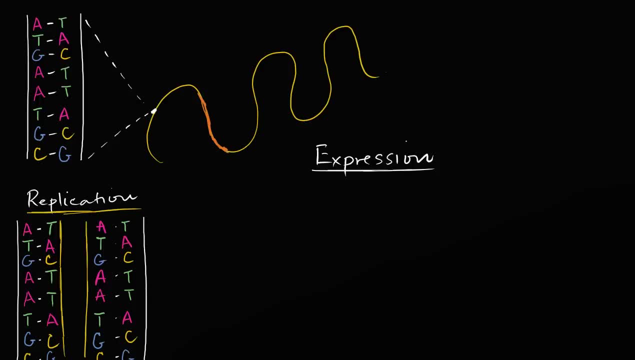 It might define. it could this information for one gene? it could define a protein. This one might- this section right over here could do- could be used to define another gene, And genes could be anywhere from several thousand base pairs long all the way up into the millions. 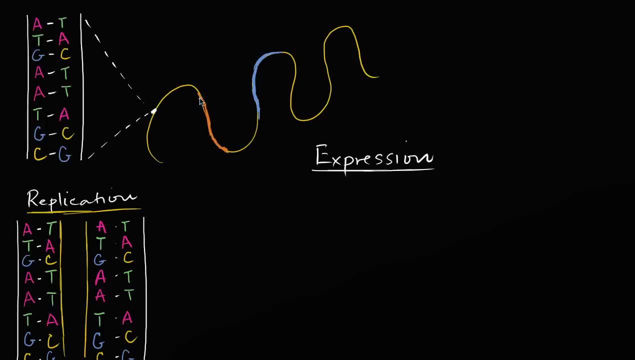 And, as we'll see, the way that a gene is expressed, the way we get from the information for that section of DNA into a protein, which is really how it's expressed, is through a related molecule to DNA, and that is RNA. 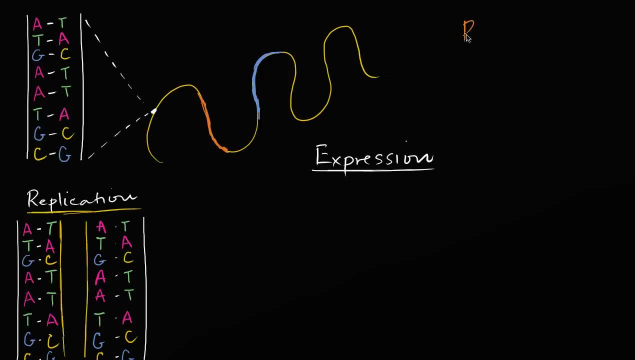 And actually let me write this down: RNA, RNA, So RNA stands for ribonucleic acid, Ribonucleic acid, let me write that down- Ribonucleic ribonucleic acid, And so you might remember that DNA is deoxyribonucleic acid. 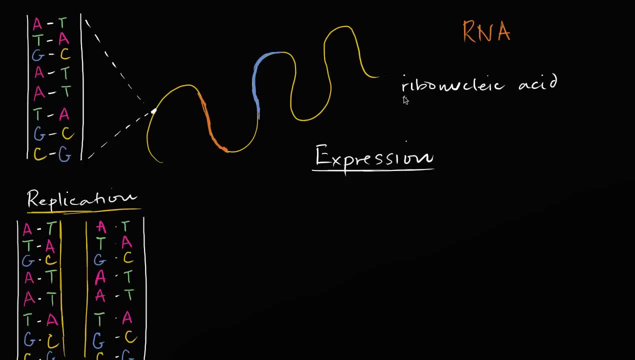 so the sugar backbone in RNA is a very similar molecule. Well, now it's got its oxy. it's not deoxyribonucleic acid, it's ribonucleic acid, The R. let me make it clear where the RNA comes from. 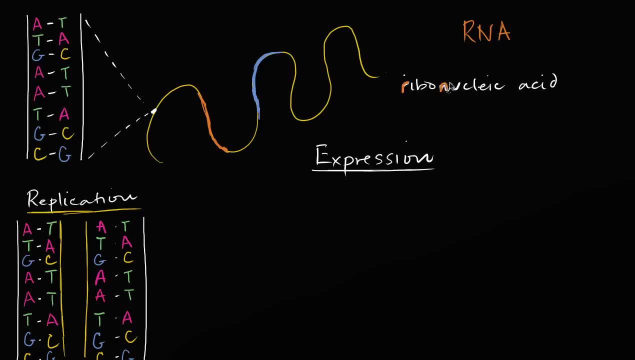 The R is right over there. You have the nucleic, that's the N. it's found well, it's nucleic and then it's A acid. Same reason why we called the DNA nucleic acid. So you have this RNA. 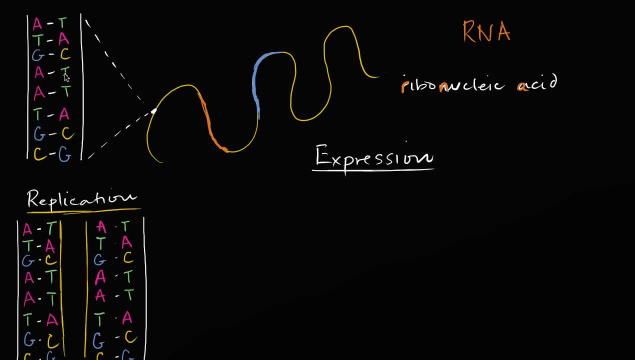 So what role does this play as we are trying to express the information in this DNA? Well, the DNA, especially if we're talking about cells with nuclei. the DNA sits there, but that information has to, for the most part, get outside of the nucleus in order to be expressed. 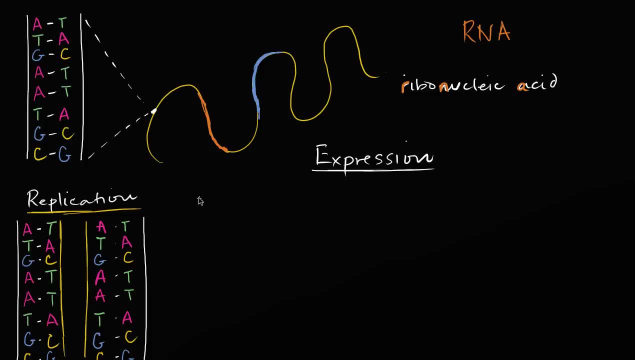 And one of the functions that RNA has is to be that messenger, that messenger between a certain section of DNA and kind of what goes on outside of the nucleus, so that that can be translated into an actual protein. So the step that you go from DNA to mRNA, 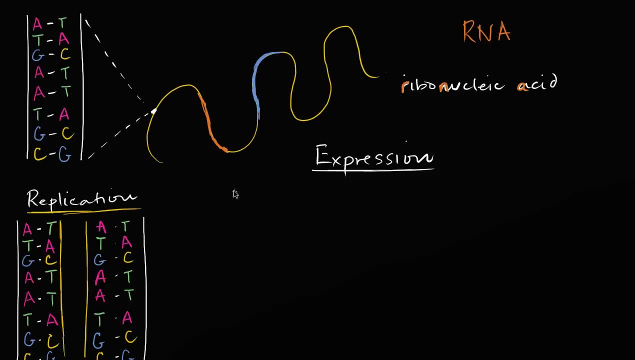 messenger RNA is called transcription. Let me write that down Transcription And what happens in transcription. let's go back to looking at one side of this, one side of this DNA molecule. So let's say: you have that right over there. 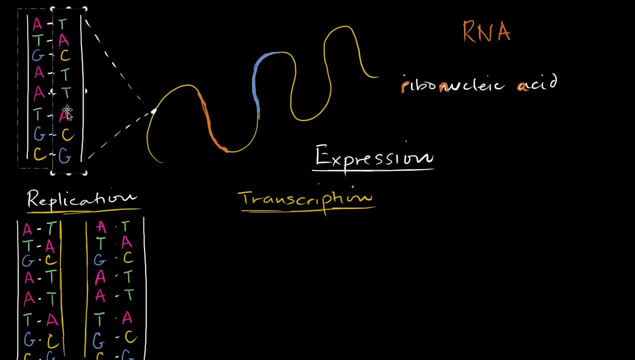 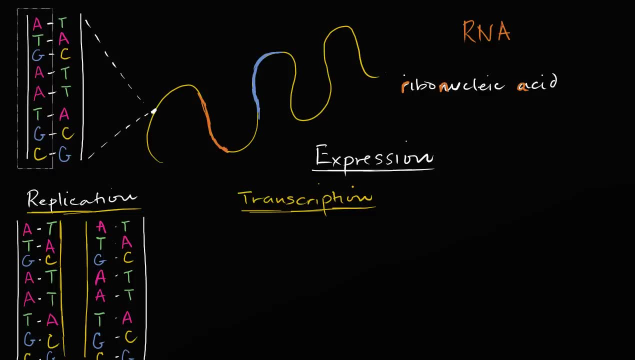 Let me copy and paste it. So there we go. Actually I didn't want to do that, I wanted the other side. So actually I think I'm on the wrong. let me go back here, And so let me copy and then let me paste. 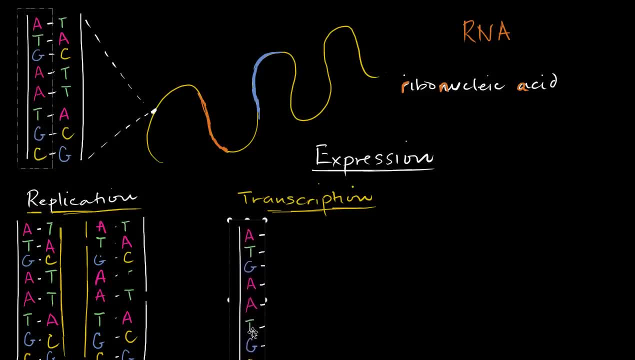 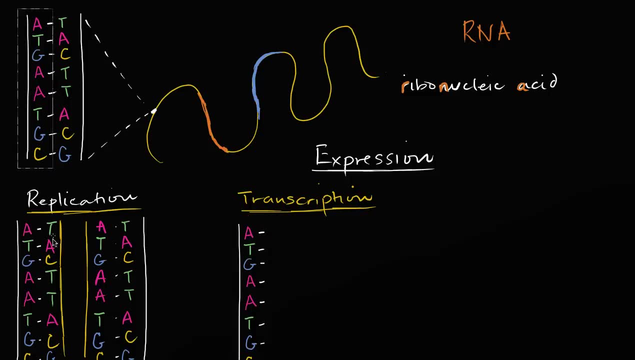 There we go. So let's say you have, let's say that you have part of this DNA molecule or you have one half of it, just like we did when we replicated it. But now we're not just trying to, we're not just trying to duplicate the DNA molecule. 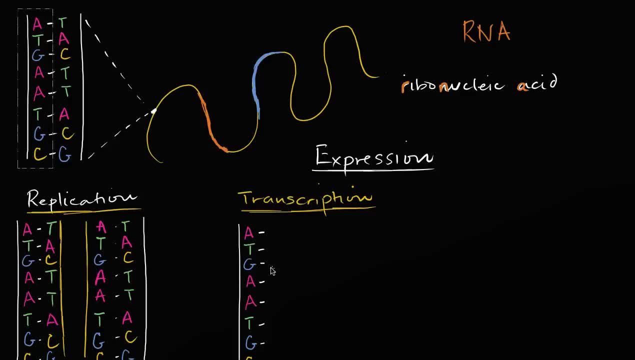 we're actually trying to create a corresponding mRNA molecule, at least for that section, that section of at least for that gene. So this might be part of a gene that actually whoops. let me make sure I'm using the right tool. 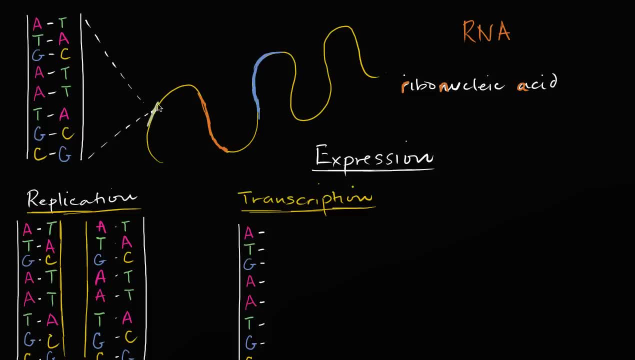 This might be part of a gene, that is, you know, this section of our DNA molecule right over there. And so transcription is a very simple, very similar conceptual idea where we're now going to construct a strand of RNA and specifically mRNA. 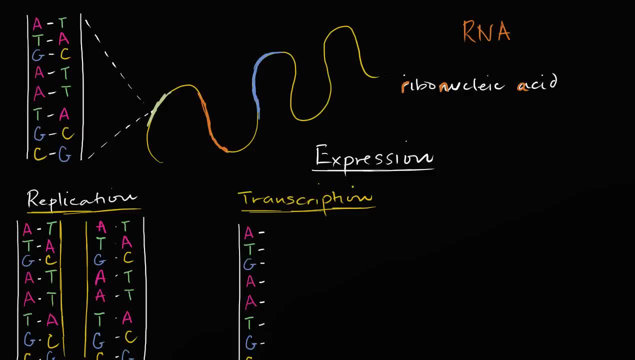 because it's going to take that information outside of the nucleus, And so it's very similar, except for when we're talking about RNA. adenine, instead of pairing with thymine, is now going to pair with uracil. So let me write this down. 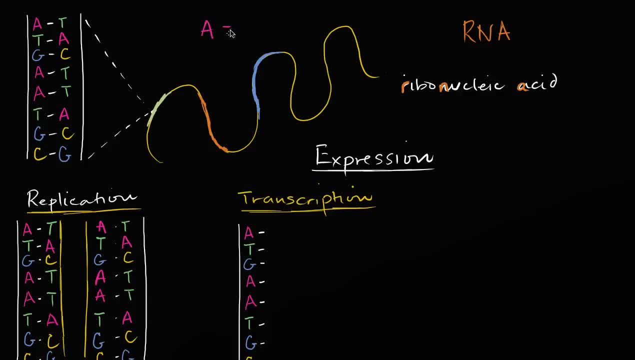 So now you're going to have adenine pairs, not with thymine, but uracil. DNA has uracil instead of the thymine, but you're still going to have cytosine and guanine pairing. So for the RNA. 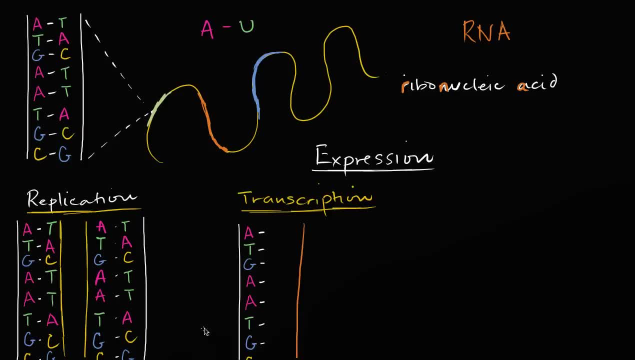 and in this case, the mRNA that's going to leave the nucleus A is going to pair with U- U for uracil. So uracil, uracil. that's the base we're talking about. Let me write it down. 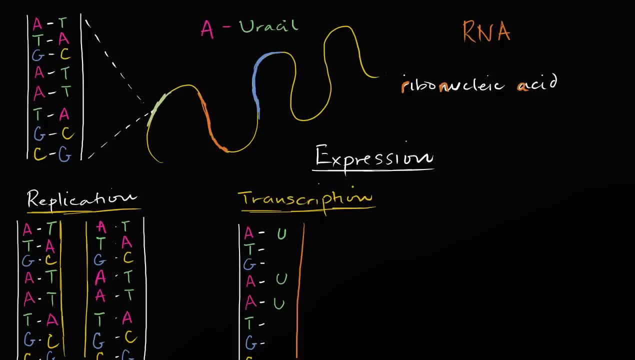 Uracil uracil Thymine is still going to pair with adenine. It's still going to pair with adenine, Just like that Guanine is going to pair with cytosine, Guanine and cytosine. 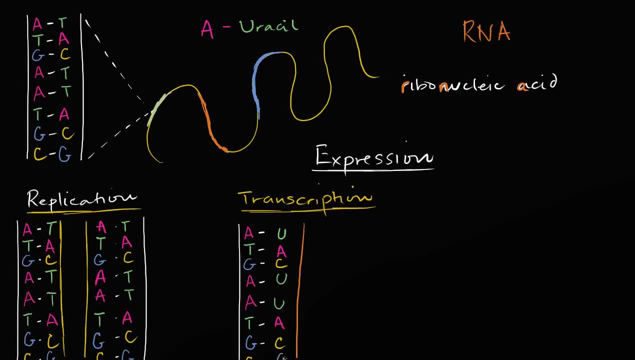 and cytosine is going to pair, cytosine is going to pair with guanine, And so when you do that, now these two characters can be attached and now you have a single strand of RNA, and in this case, messenger RNA, that has all the information. 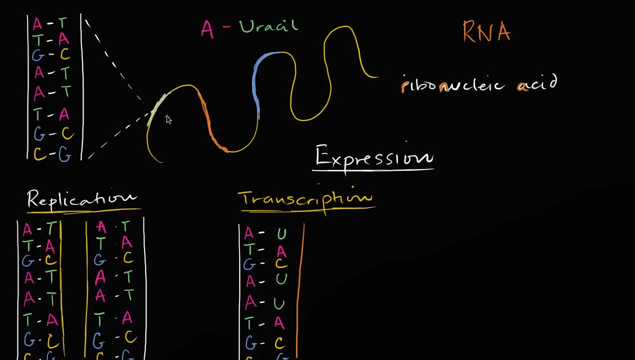 on that section of DNA, And so now that thing can leave the nucleus, go attach to a ribosome- and we'll talk more about that in future videos, exactly how that's happened- And then this code can be used to actually code for proteins. 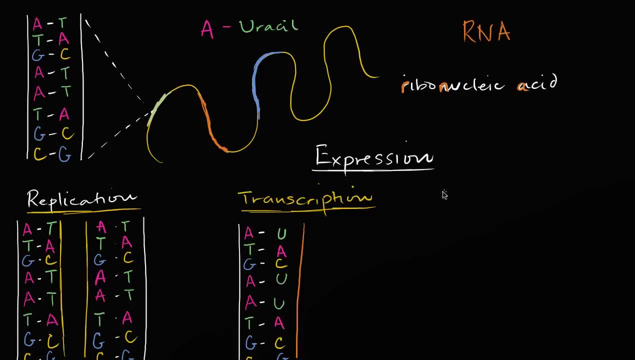 Now, how does that happen? And that process is called translation. So translation. Translation, Which is really taking this base pair sequence and turning it into an amino acid sequence. Proteins are made up of sequences of amino acids, So translation. So let's take our mRNA. 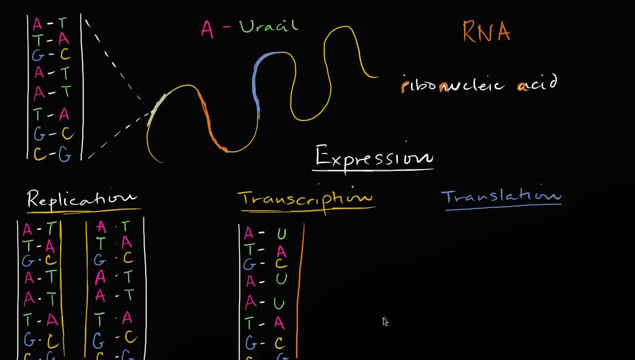 or this little section of our mRNA, and actually let me do it, let me draw it like this, Let me draw it like this And let's see I have it is UAC, so it's going to be UAC. 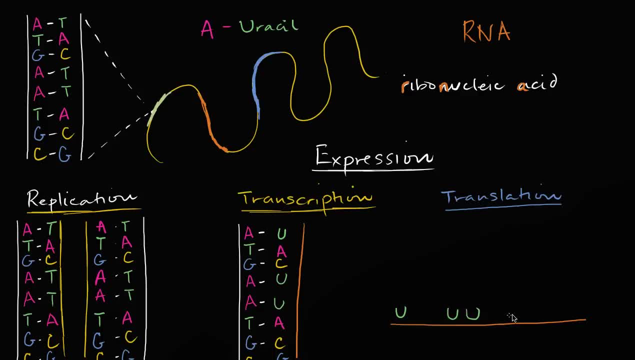 then UU, then ACG- okay, And then we have an A. let me make sure I change to the right color. we have an A there, and then we have this UUACG. alright, now let me put a C right over there. 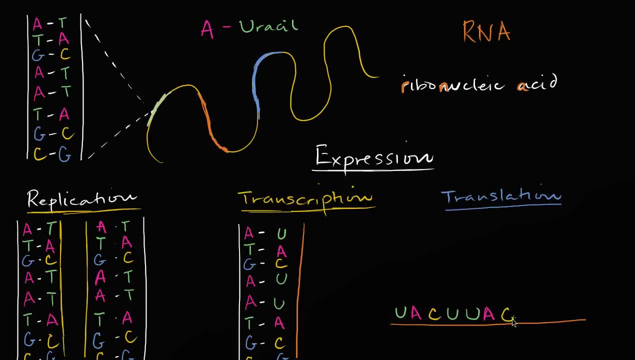 I'm just taking this and I'm writing it horizontally: I have a C here, not a G, it's a C, And then, finally, I have a G, And of course it'll keep going on and on and on, And what happens is: 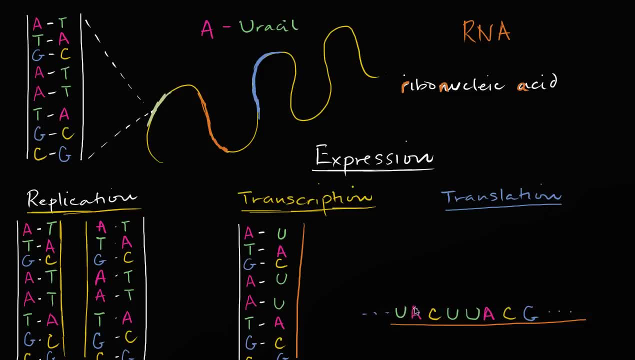 each sequence of three, and you have to be very careful where it starts, and so this is in some ways a delicate and surprising but at the same time surprisingly robust process. every three of these bases code for a specific amino acid, And so three bases together. 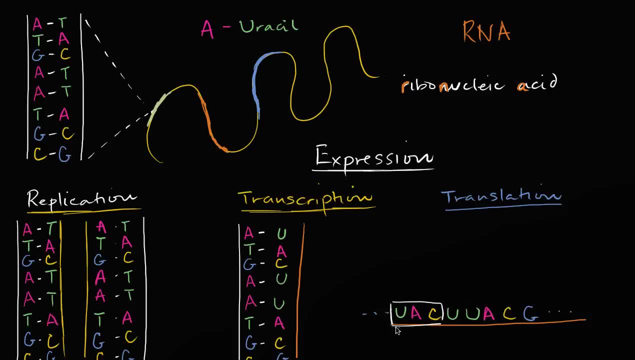 so these bases right over here, I guess you could say this three letter word or this three letter sequence, that's called a codon, Codon, And this is going to be the next codon, The next codon, And we actually haven't drawn the next codon after that. 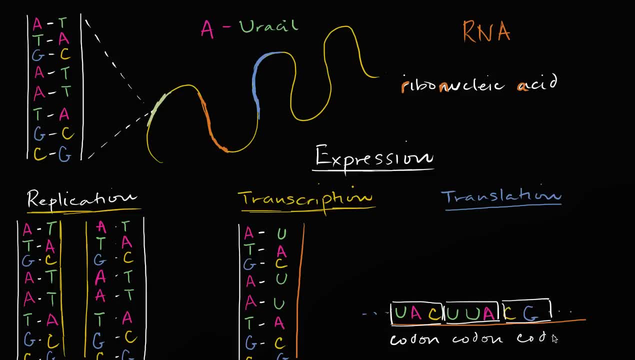 because we need three bases to get to the next codon. And how many possible codons do you have? Well, you have one of four bases and you have them in three different places. so you have four times four times four possible codon words. I guess you could say: 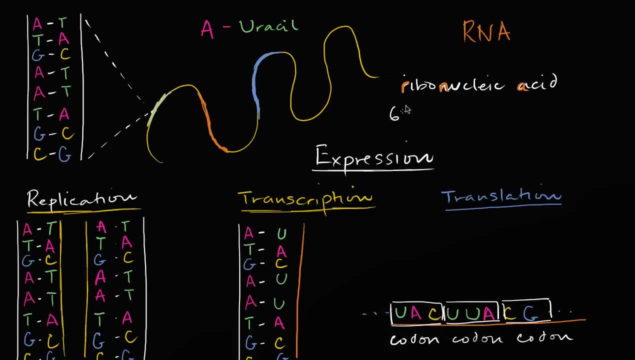 and four times four times four is 64. So you have 64 possible codons, which is good because you have 20 possible amino acids. So this is overkill and it allows codons to be used for other purposes as well. 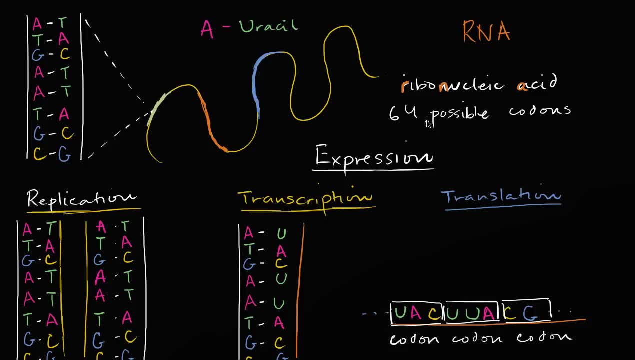 and they also. you know you might have more than one codon coding for the same amino acid, So you have 64 possible codons. they need to code for 20 amino acids and so this codon right over here with the ribosome. 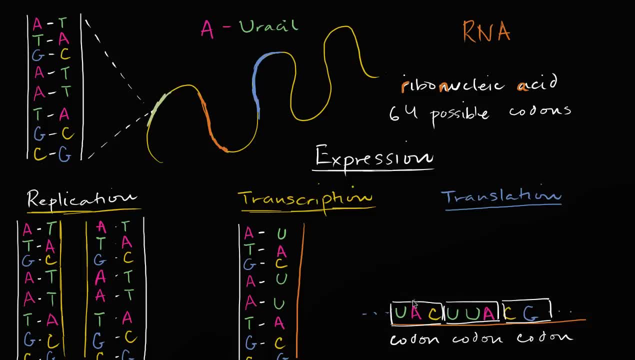 and we'll talk more about how that happens. can code for. can code for, say, could code for amino acid one? So let me just write it here: This is amino acid one, And actually this amino acid is brought to here. 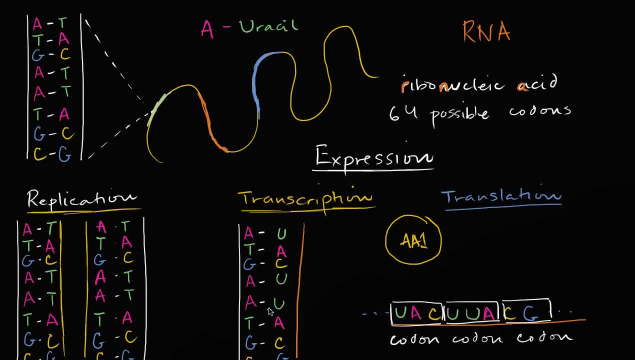 They're actually matched together by another type of RNA. This is mRNA we're talking about right over here. This is mRNA, But there's another type of RNA called tRNA that essentially- that essentially- brings these two characters together. So the tRNA- and I'm just gonna you know. 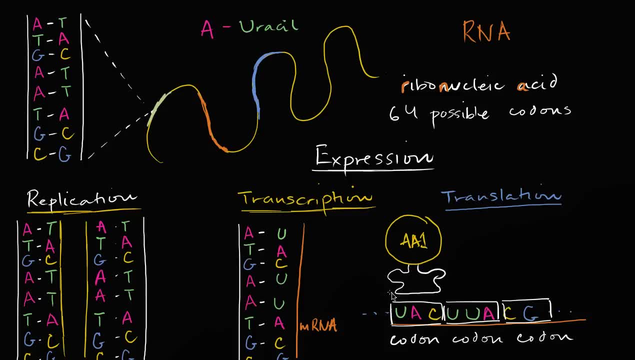 it's got some structure here. I'm not drawing it completely right, but it's going to match right over here where maybe it has. it has an A, a U and a G right over here and on this end it was attached to this amino acid. 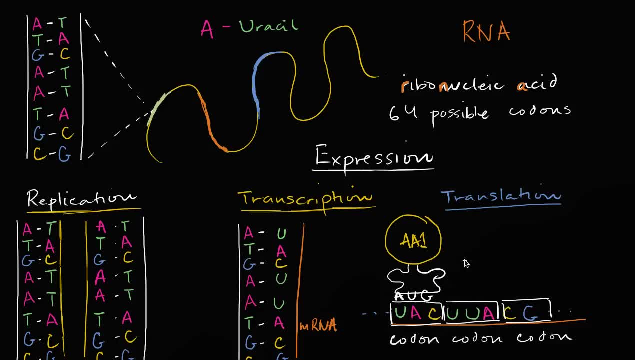 and so it matches them together, And then you're gonna have another, another tRNA that might attach to amino acid two, which I will do in purple amino acid two, and that just happens to coincide with, so it can complement right over here. 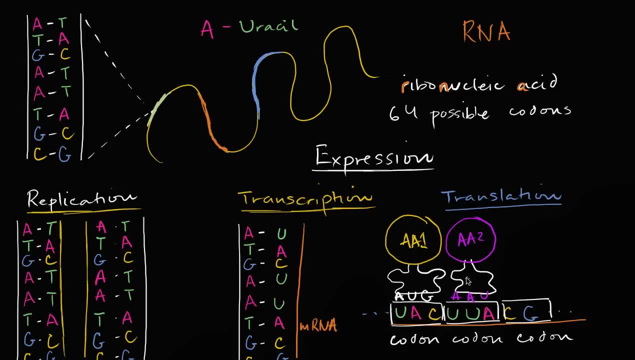 so it attaches in the right place. so it's A, a U right over here, this tRNA, and so it'll construct the sequence of amino acids, And as you put these amino acids together, then you are actually constructing a protein.